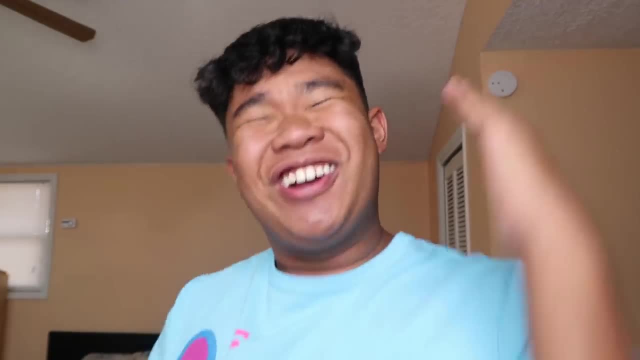 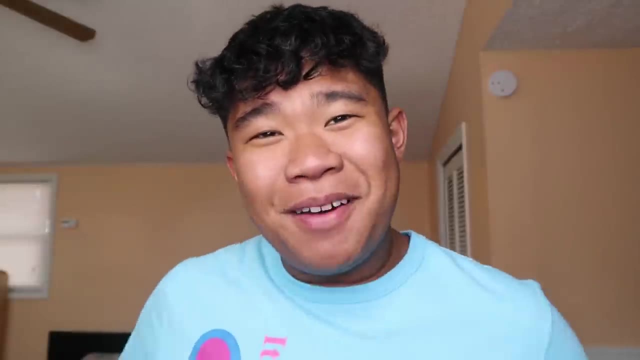 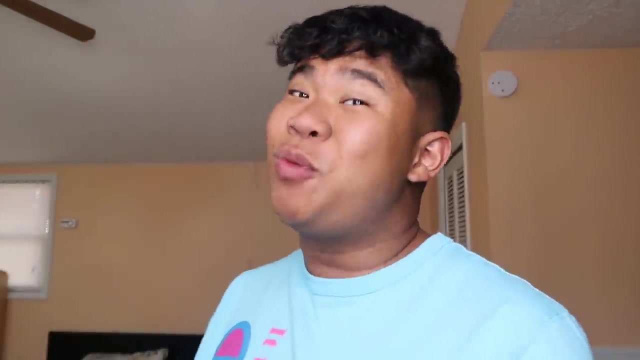 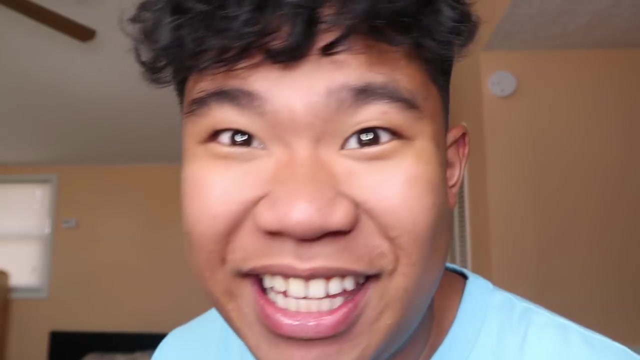 If you're new to this channel, make sure you hit that subscribe button down below. We're slowly growing on YouTube, man. It makes me so happy, bro. Fun fact, I started on YouTube before I was doing TikTok. So like, hit that subscribe button, man. Support your boy's dreams. TikTok might be banned soon, So I need all the support that I can get. Make sure you hit that notification bell as well, so you never miss an upload. But anyways, with that being said, let's get right into the world's most easiest self-working- no set of nothing card trick. That made it sound lame, It's cool, I promise. All right, So I'm about to show you the easiest self-working card trick. 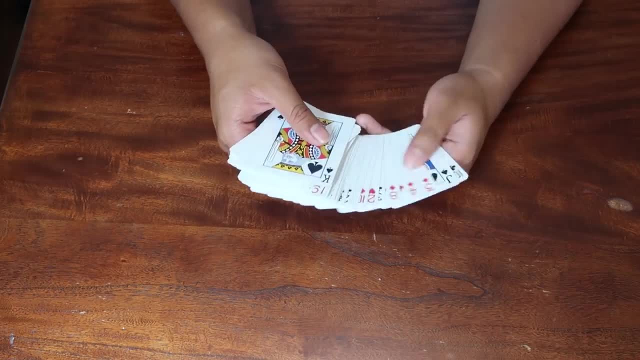 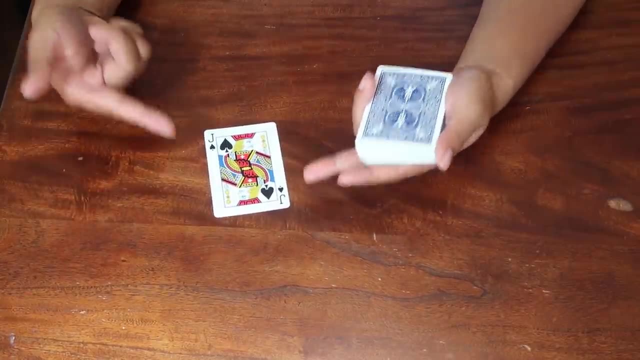 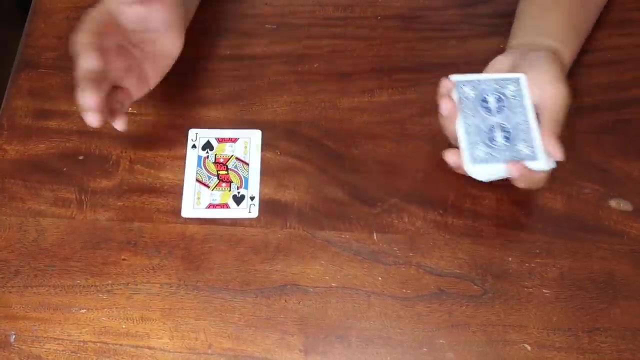 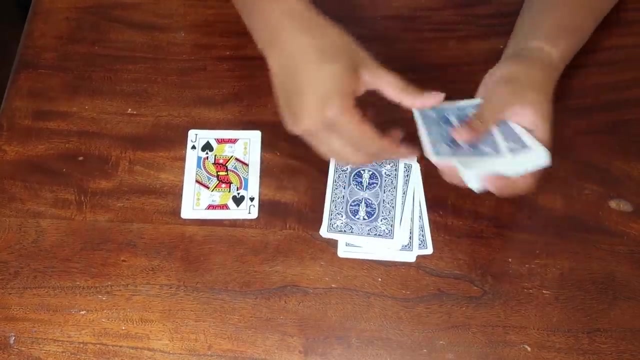 Ever And it goes with a little bit of a storyline. So for this we're going to need the Jack of Spades. This is a little bounty hunter. Yes, we got a little story about Jack the bounty hunter. This Jack can find any criminal, any card in the deck of cards, And I'll prove it to you right now. For this we're going to need a shuffle deck of cards and we're going to need two piles of 15.. So let's count it out: 1, 2,, 3,, 4,, 5,, 6,, 7,, 8,, 9,, 10,, 11,, 12,, 13,, 14, 15.. 1,, 2, 3, 4, 5, 6,, 7,, 8,, 9,, 10,, 11,, 12,, 13,, 14, 15.. 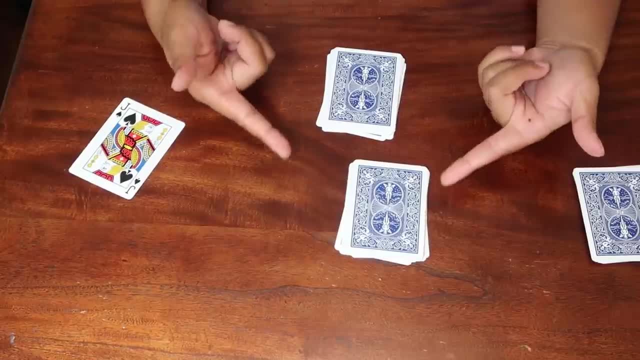 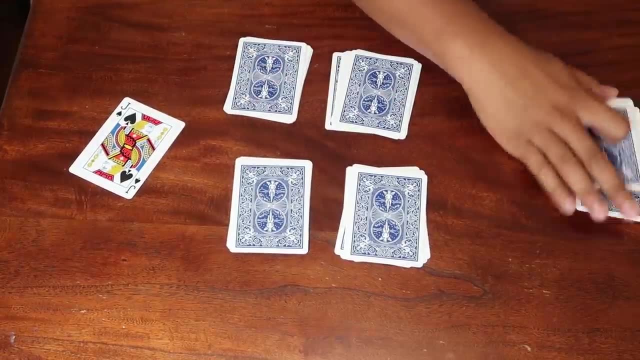 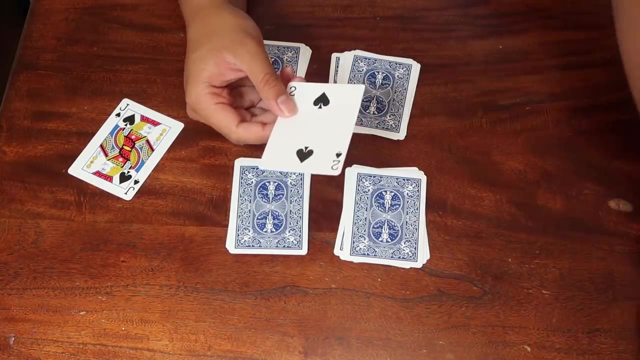 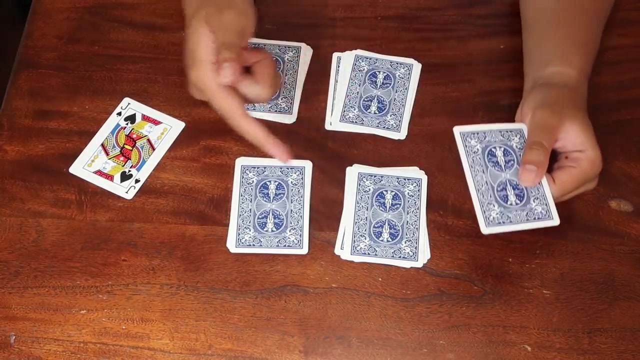 All right, Cool, Now that you've got two piles, I'm going to ask the spectator: hey, with your pile, go ahead and cut it wherever you want. So the spectator cuts it wherever they want. With my pile, I'm going to go ahead and cut it wherever I want. And with the remainder of the cards, we need a criminal. So we're going to pick one, And the spectator can pick any card they want. In this case, we've got the wanted two of spades. Oh, the baddest criminal on the planet. You're going to say, hey, spectator, your wanted two of spades. Go ahead and point to any pile. So, whichever pile that they want to put it on top of, they can. All right, So they. 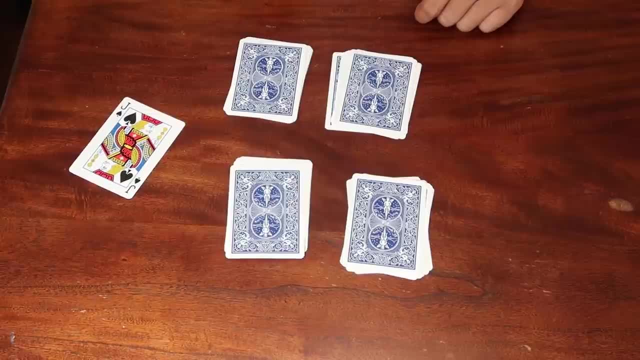 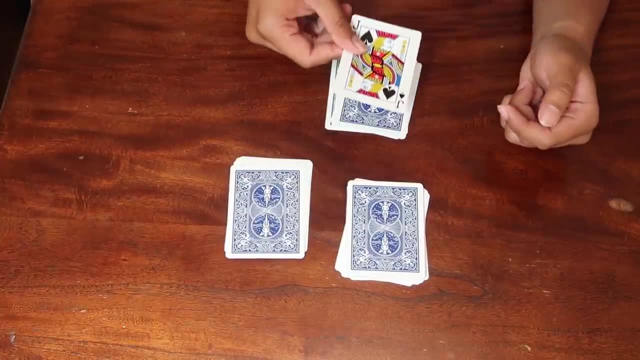 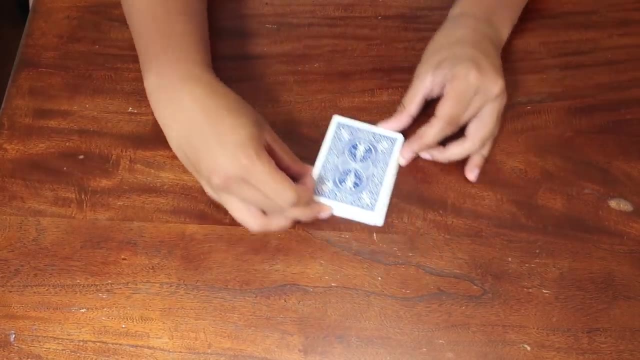 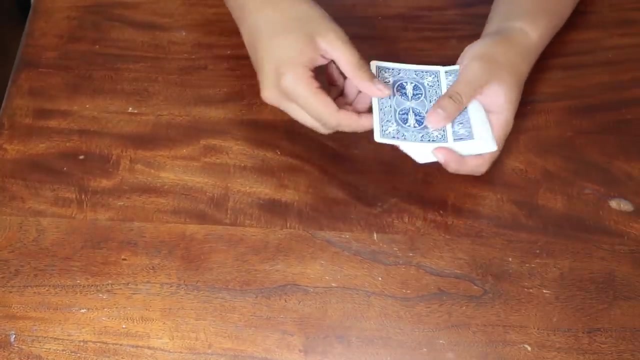 put on there and point to one of my piles to lose that card in the middle. So they can choose either pile. So say this one, right here, Bam, Their card is now lost, And the same thing goes with the jack. The jack goes on my last pile And the pile that they did not select. we'll lose it right there And then we'll just stack these two together, just like so. So not only is your card lost, the jack, the bounty hunter is also lost. But guess what? It can hunt down any card. Because look, if you just start dealing through it like so into two piles, you'll notice the jack. 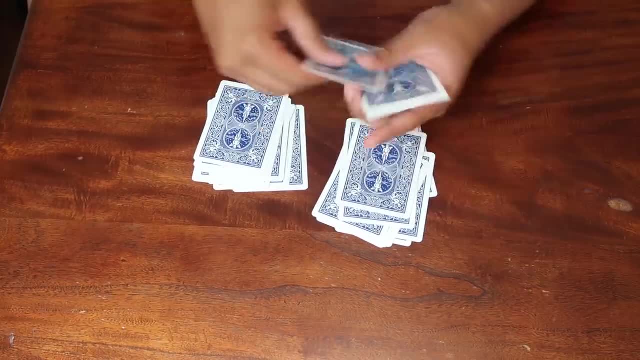 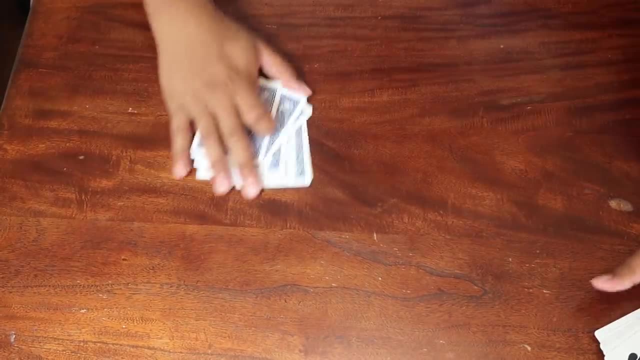 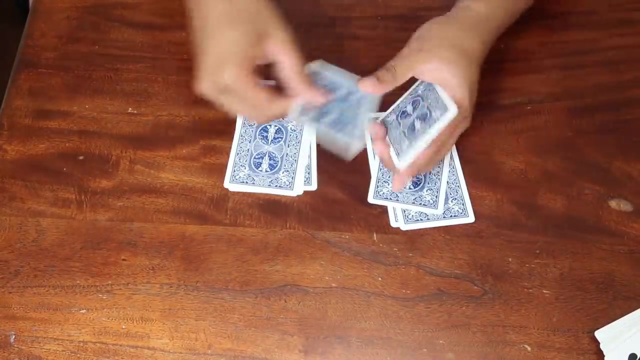 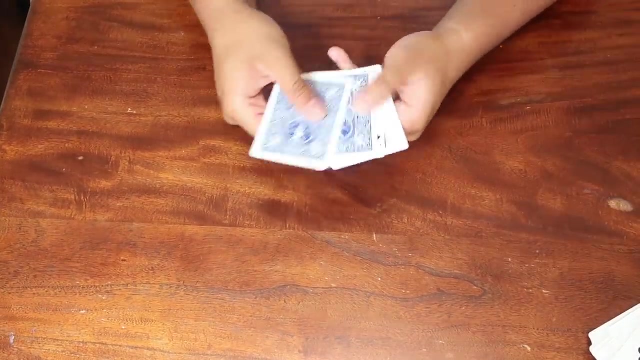 starts to weave through all the criminals, through all of the suspects. slowly and surely There's a first one. Look, the jack is not in this pile, So we're going to remove this pile. And he still thinks that some people might hear might be a little suspicious. All right, So we're going to keep dealing through it. Okay, The jack is looking through more suspects. Jack isn't in this pile, So we're going to remove those. Huh, There's a few more suspects going through here. We're going to keep dealing. No, 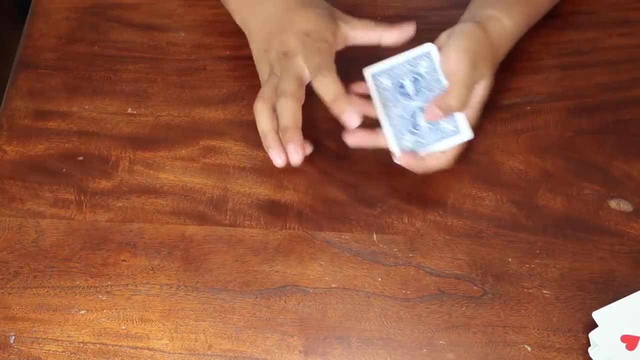 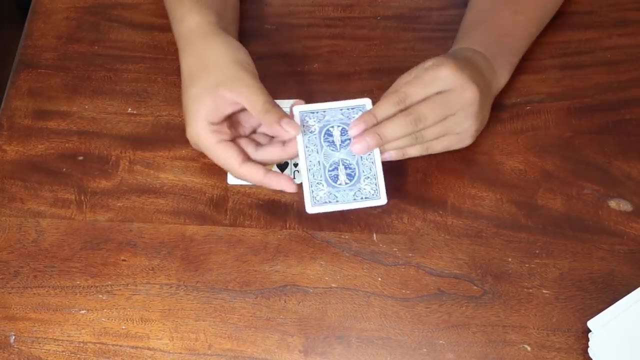 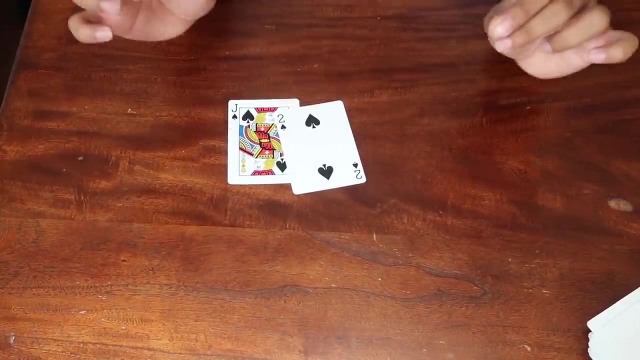 jack in here. We're going to remove that And we got a few left And we just deal it one last time. We'll remove these And the jack seems to have found one card and one card only. You're two of spades, the criminal Dang. that is so cool. Literally the coolest card trick ever. 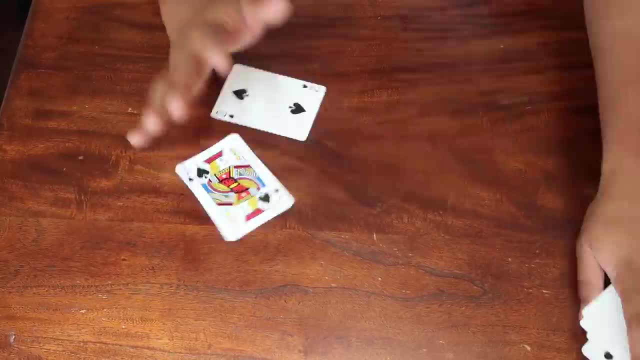 Fooled me And guess what? There is literally no tutorial. Okay, That's a little bit of an exaggeration, but there's basically no tutorial Because you just have to follow exactly what I did in this video And I'm going to show you how to do it. So let's get started. 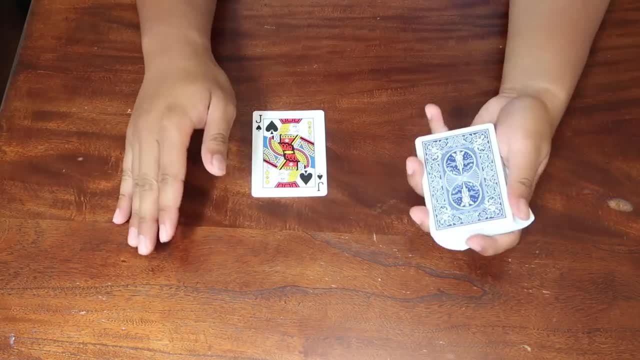 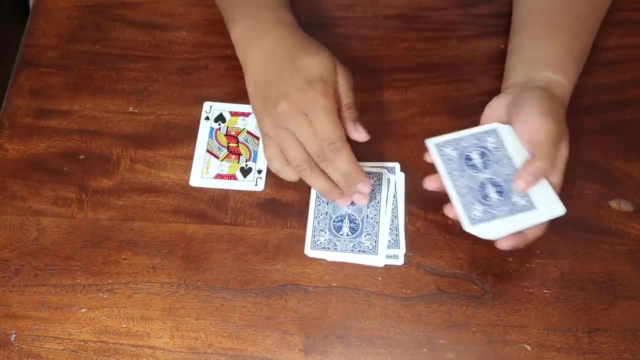 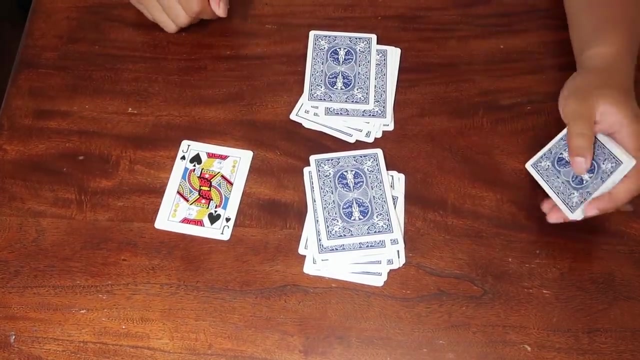 And you will, 1 million percent of the time, all the time, find the card. So to break it down, just so you know what to do, you basically want two piles of 15.. So here's four, And of course you need the jack, And what you do is you ask the spectator to cut their pile. So 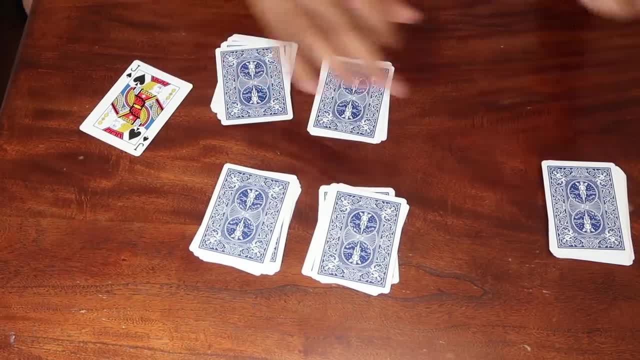 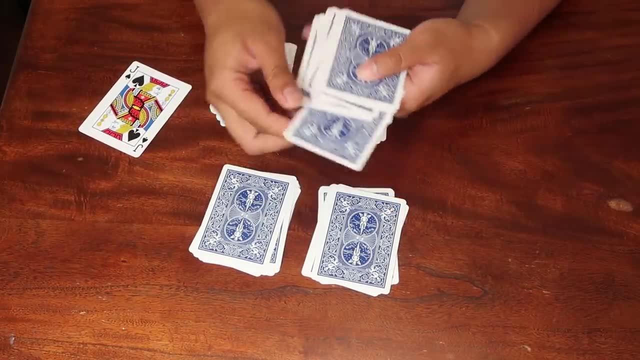 this is their pile into two. You cut your pile into two With the remainder of these cards, the ones that you didn't deal out, nor the jack. make sure you have them. just pick any card and memorize it. So in this case, we got the 10 of clubs You're going to say. 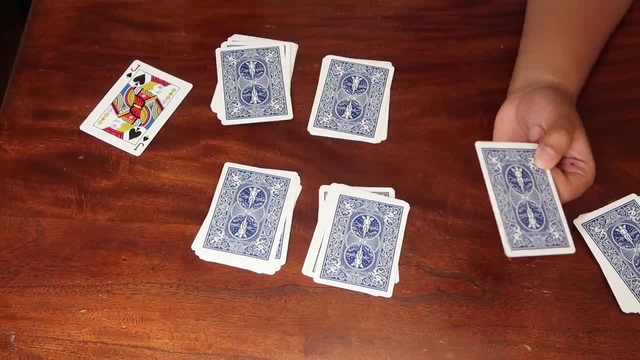 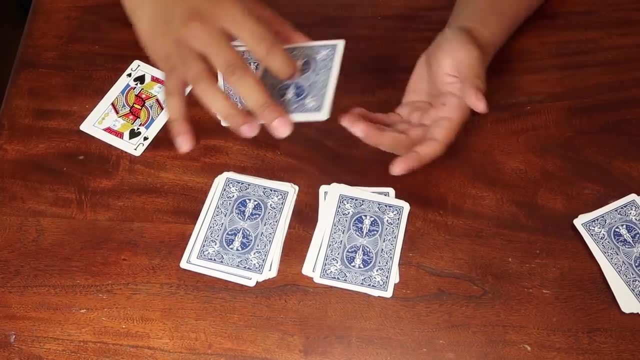 whatever card that they picked, it's a criminal. And you ask them to put it on top of any one of these piles, So they can literally put on top of any one of these piles. You ask them to pick one of your piles so they can place it on top of the stack. Literally, you're just following exactly. 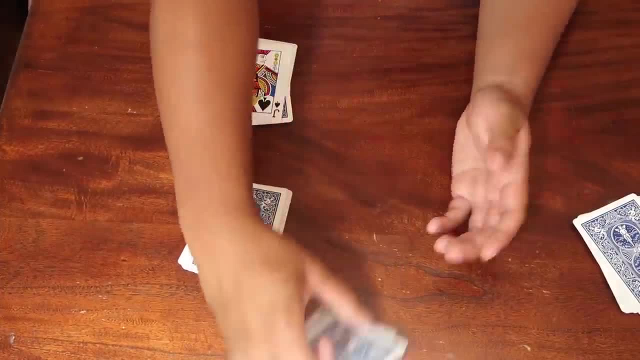 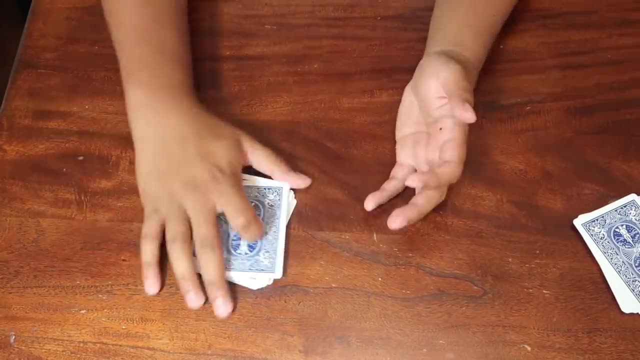 what I did earlier. You take the jack, leave it face up and take the other pile on their side and then put it on top. And then you want to take the pile with the jack and place it on top of the pile with the card.